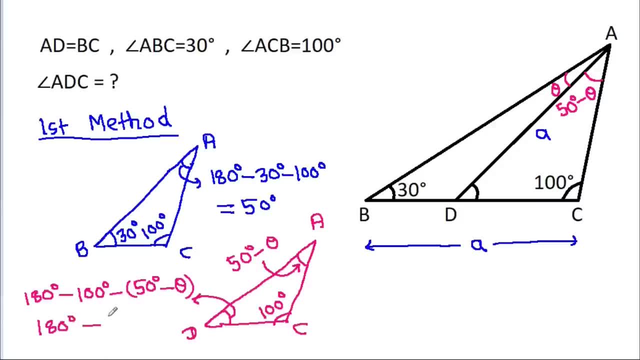 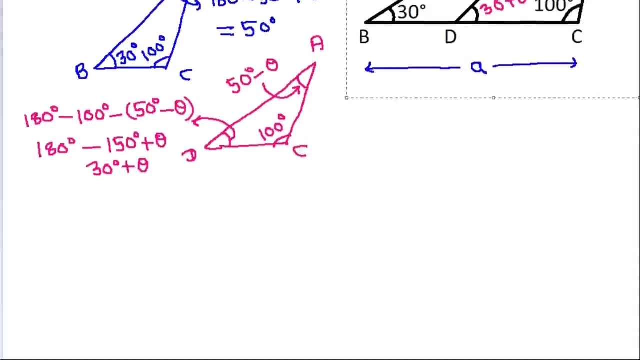 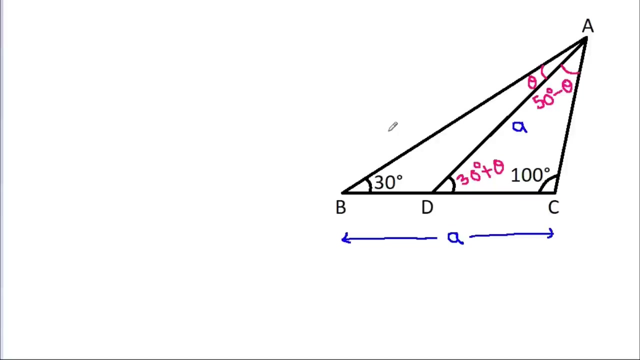 it is 180 degree minus 150 degree minus theta, that will be 30 degree minus theta. so this angle, it will be 30 degree minus theta. and now in any triangle, A, B, C, if BC is A, AC is B and AB is C, then A by sine, A it is. 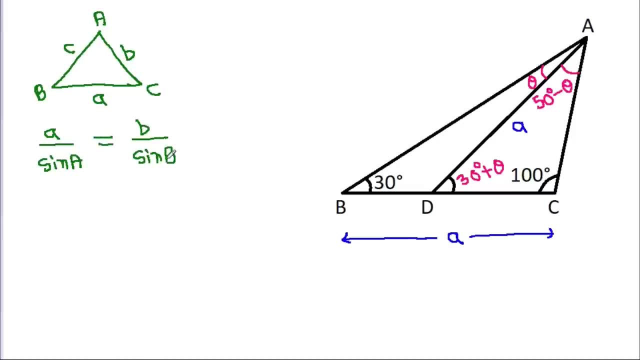 equal to B by sine B, it is equal to a, b, a, C by sin C. and here suppose AC is B, then inter angle ABC, it is A, B, C, B, C, C, B, C is A and AC is B, and this angle it is 50 degree and this angle it is 30 degree. 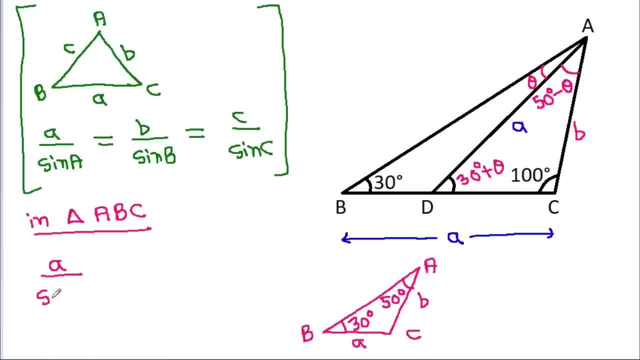 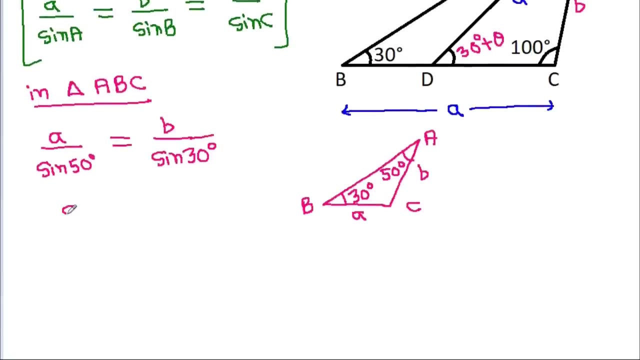 So A by sin 50 degree, it will be equal to B by sin 30 degree. So A by sin 50 degree, it will be equal to B by sin 30 degree. So A by B, it will be equal to sin 50 degree by sin 30 degree. and. 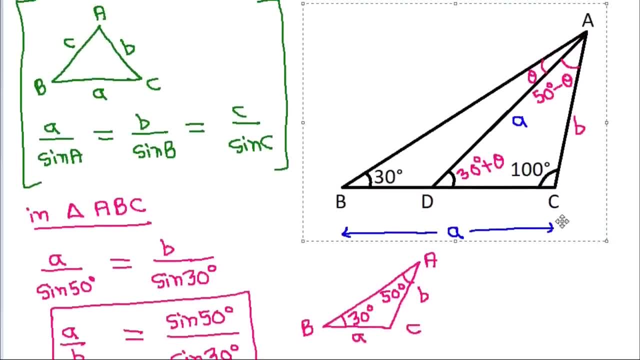 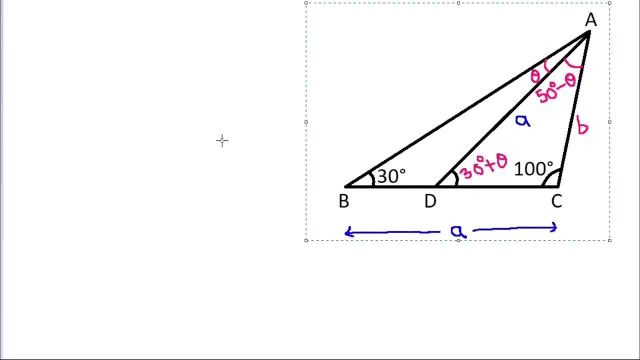 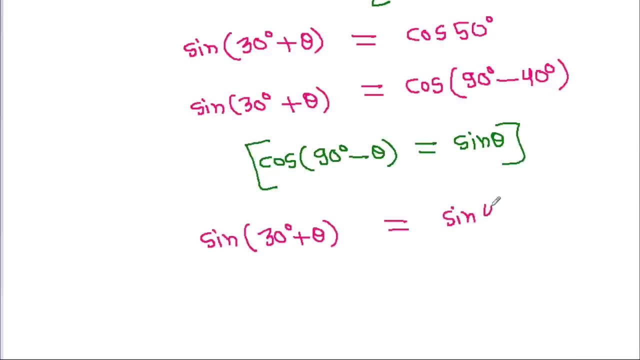 So A by sin 30 degree, it will be equal to B by sin 30 degree, equal to sine 40 degree. so 30 degree plus theta it will be equal to 40 degree. that means theta. it will be equal to 40 degree minus 30 degree, that is 10 degree. 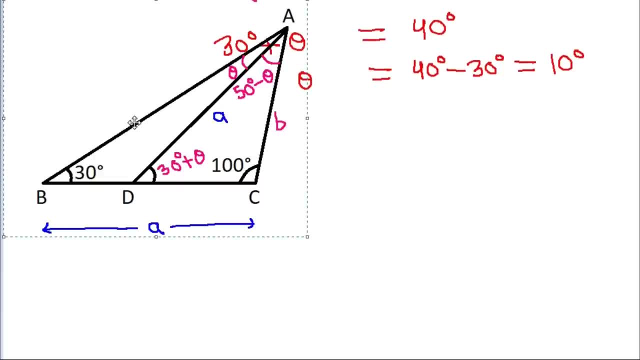 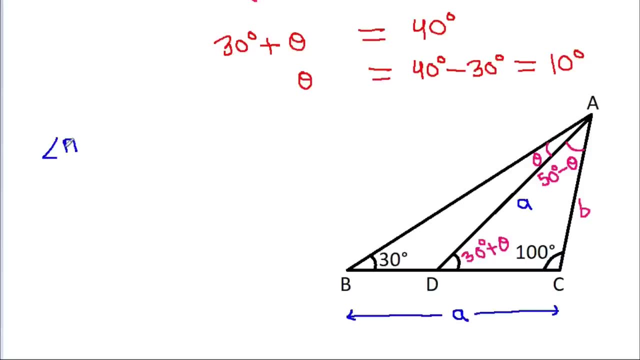 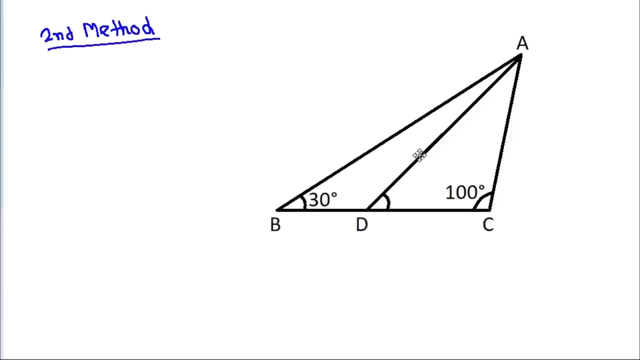 and now angle ADC, it is equal to 30 degree plus theta, that will be equal to 30 degree. plus 10 degree, that will be equal to 40 degree. and second method we have: AD is equal to BC. so if AD is A, then BC it will be A. 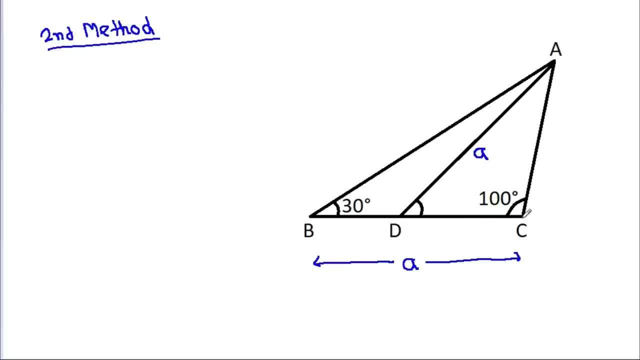 and now, if we extend BC and draw a perpendicular from A to BC, suppose this point IS E, suppose this angle IS theta, and suppose CE is X and AE is c its c isassen, and suppose CE is x and AE is c itssen, and suppose CE is x issen. 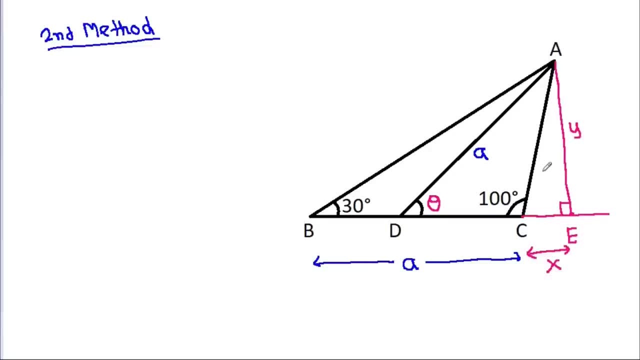 and suppose CE is x, issen, and suppose this angle IS theta, and suppose CE is x and AE is 7 is y, then this angle here we have. this angle is 100 degree, so it will be 180 degree minus 100 degree, that will be 80 degree, so it will be 80 degree. so inter, 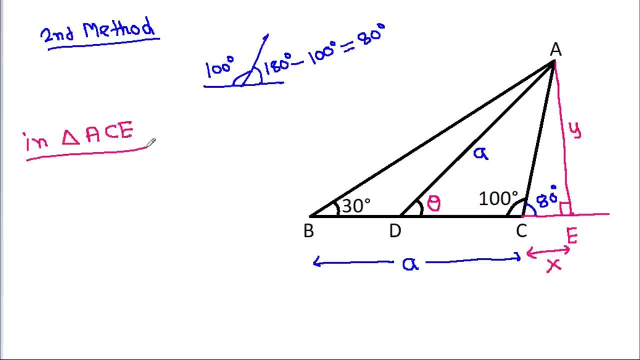 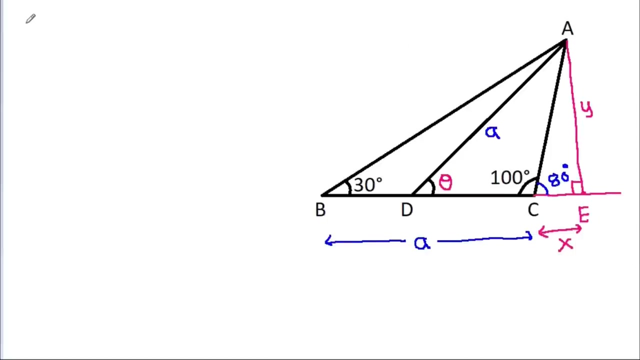 angle ACE tan 80 degree, it will be equal to AE by CE. that is equal to Y by X. so Y will be equal to X times tan 80 degree and now we have Y is equal to X times tan 80 degree and inter angle AD by Z. 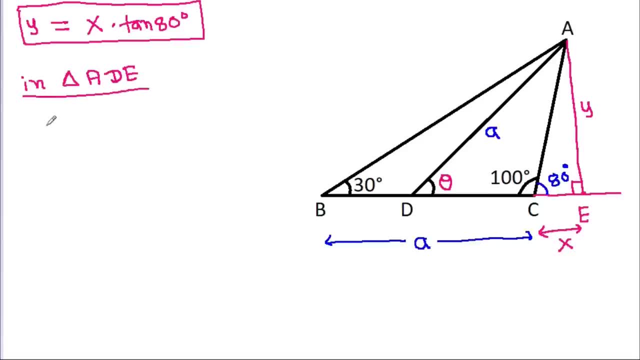 sine theta, it will be equal to AE. by AD, that is equal to Y by A. so sine theta, it is equal to Y. it is x times tan, 80 degree by A. so A will be equal to x times tan, 80 degree by sine theta. and. 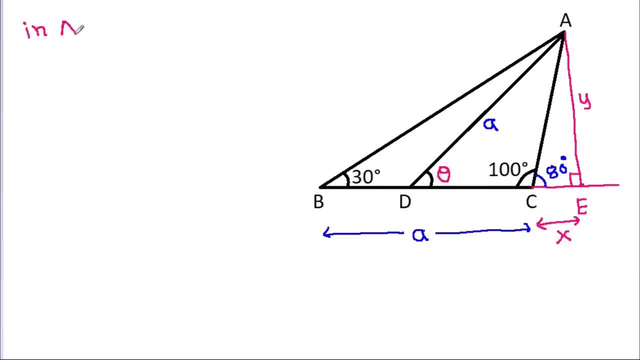 now inter angle: ABE: tan 30 degree, it will be equal to AE by BE and AE is Y. by BE it is A plus x and tan 30 degree. by sine theta it will be equal to x times tan 30 degree by sine theta. OK. 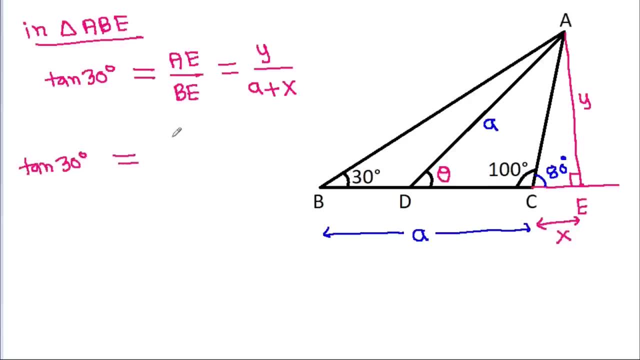 inter angle ABE. tan 30 degree, it is equal to Y. it is x times tan 80 degree. by A, it is x times tan 80 degree. by sine theta plus x and tan 30 degree, it is 1 by a square root of theta that is equal to tan 80.. 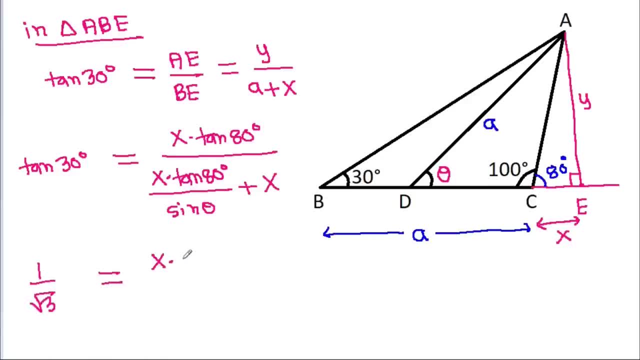 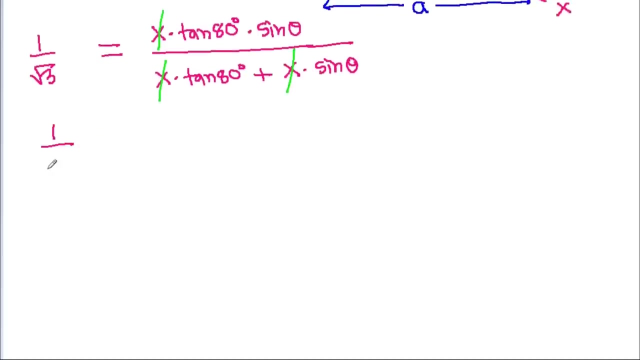 And the receive x times tan 80 degree times sine theta by x times tan 80 degree, plus x times sine theta, and x will get cancelled. And so 1 by s square root of 3, it is equal to tan 80 degree times sine theta by tan 80. 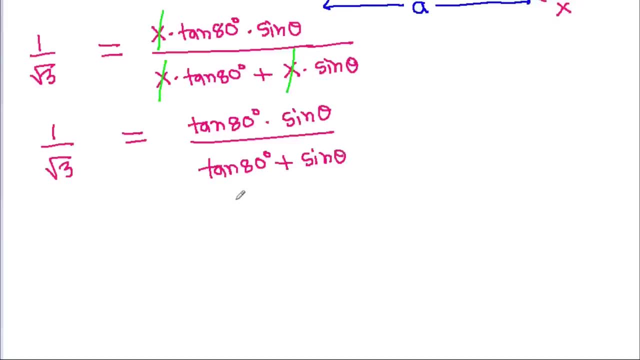 degree plus sine theta. And if we cross multiply, then tan 80 degree times sine theta is equal to tan 80 degree plus sine theta. it will be equal to s square root of 3 times tan 80 degree times sine theta. And tan 80 degree, it is equal to s square root of 3 times tan 80 degree sine theta minus. 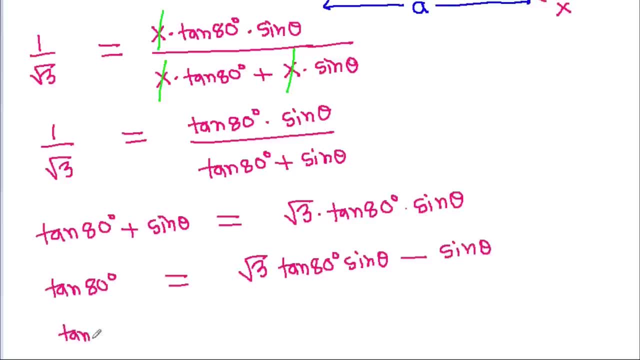 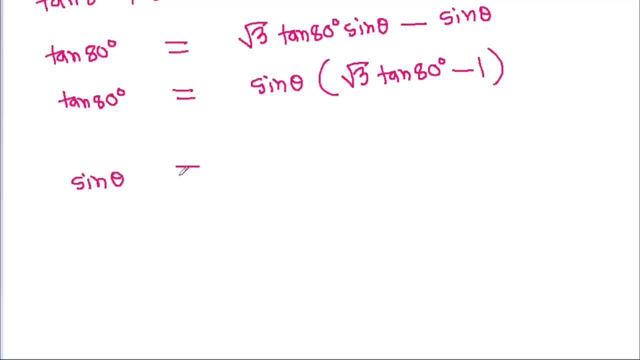 sine theta, So tan 80 degree, it is equivalent to sine theta times s square root of 3 times tan 80 degree minus 1.. So times sine theta will be equal to tan 80 degree by sine theta, And this will be given by tan 80.. 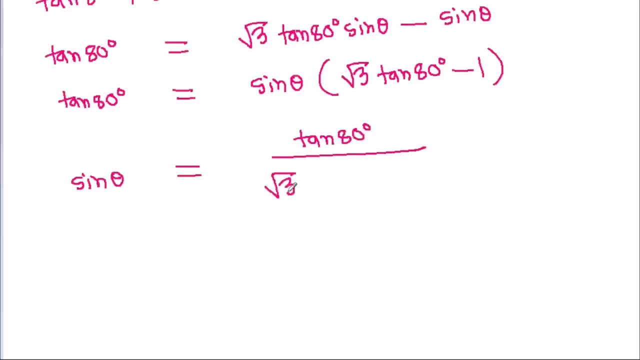 And by tan 80, it will be equal to s square root of 3 times tan, 80 degree minus 1.. So sin theta times sin theta must be equal to sine theta times s square root of 3, The square root of 3 times tan, 80 degree minus 1. and now, sine theta, it is equal to: 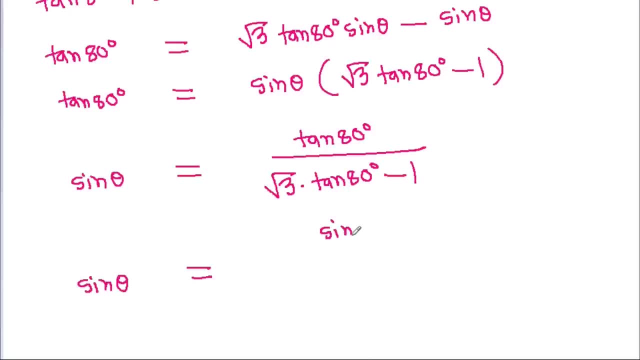 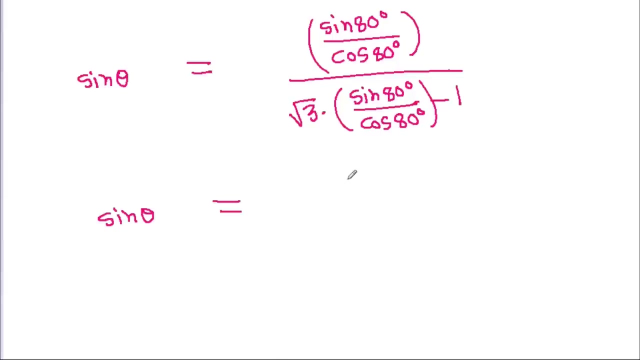 tan 80 degree, it is sine 80 degree by cos 80 degree, by a square root of 3 times sine 80 degree by Cos 80 degree minus 1, and sine theta, it is equal to sine 80 degree by cos 80 degree by square root of 3 times. 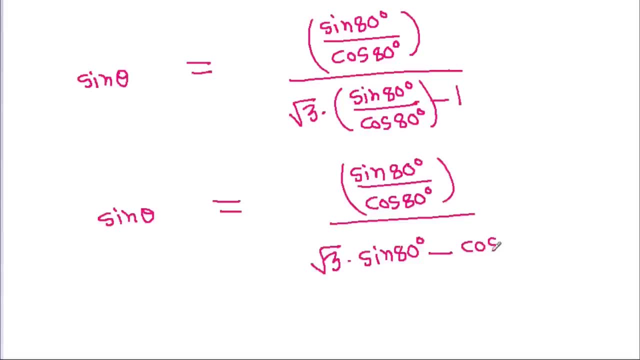 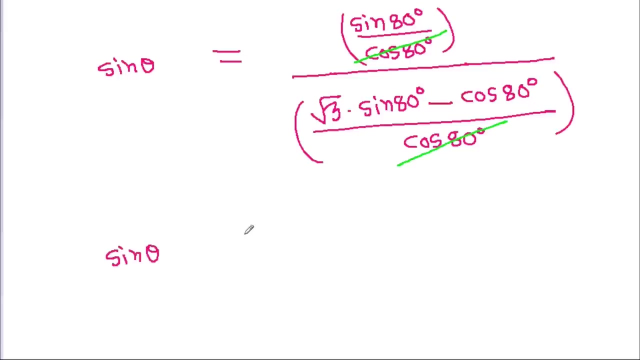 sine 80 degree by Cos 80 degree minus 1, and sin 80 degree minus cos 80 degree by cos 80 degree, and cos 80 degree will get cancelled. so, sine theta, it is equal to sine 80 degree by s square root of 3: sine 80 degree minus cos 80 degree. 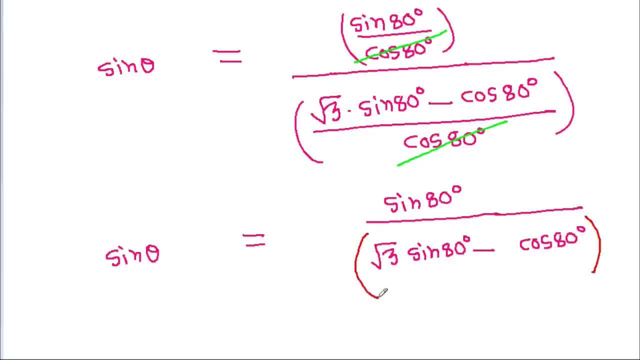 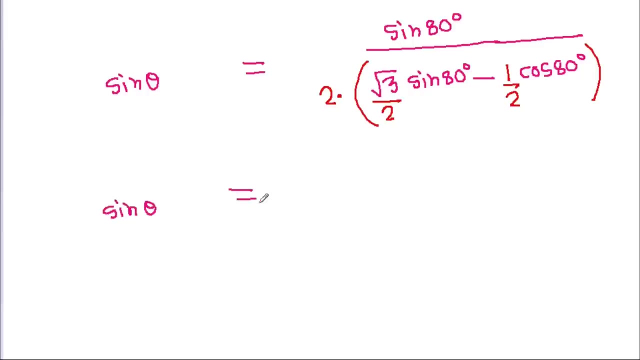 and now here, if we multiply with 2 and divide with 2, then sin theta it is equal to sin 80 degree by 2 times sin 80 degree times a square root of 3 by 2 it is cos 30 degree minus cos 80 degree times, and 1 by 2 it is sin 30 degree.